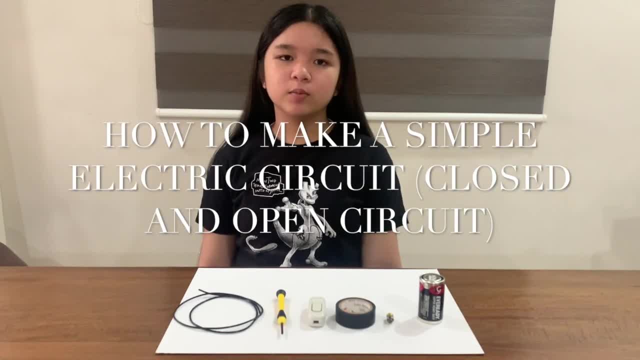 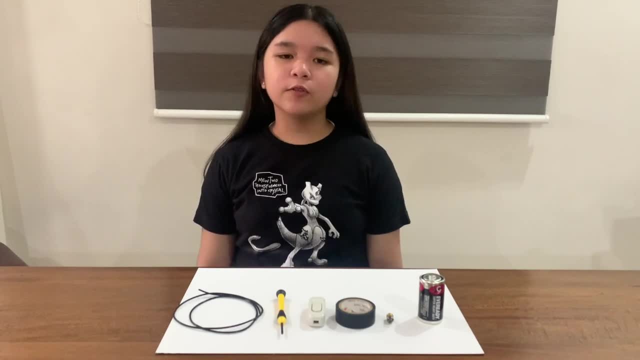 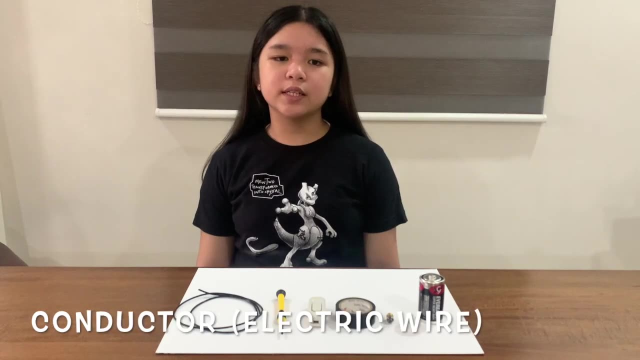 A simple electric circuit is a closed loop or a continuous path over which electrons move. It consists of the following components: First, an energy source to get the electrons move, like a battery. Second, the conductors which serve as a path along which the electrons can travel, like electric wires. 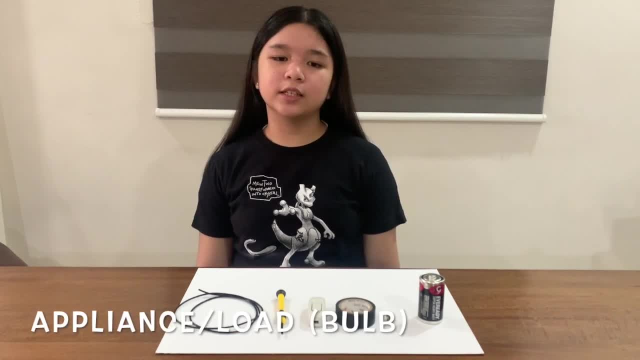 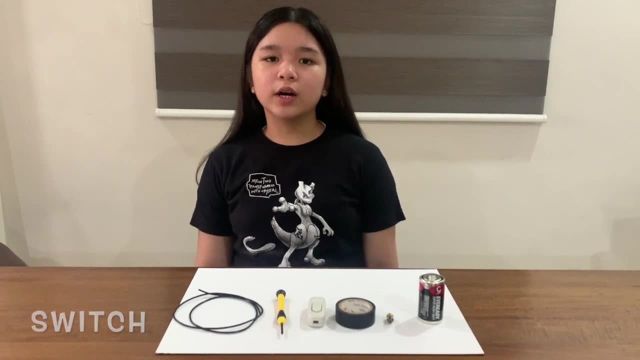 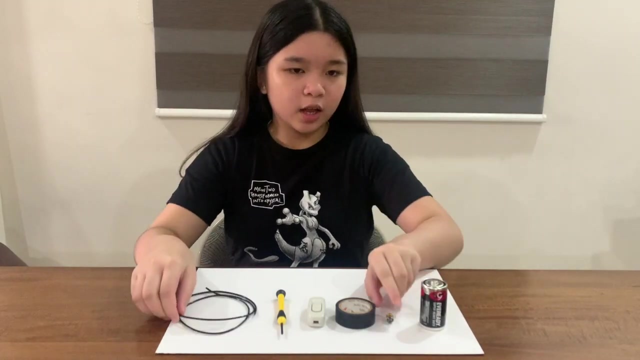 Third, an appliance or load that uses the electrical energy like a bulb. Fourth, a switch for turning on and off, like a paper clip or alligator clip. Today I am going to show you how to make a simple electric circuit. For this project we need a battery, an electric wire, a bulb and a switch. 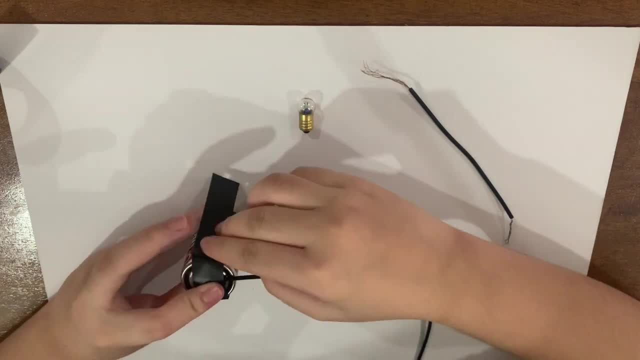 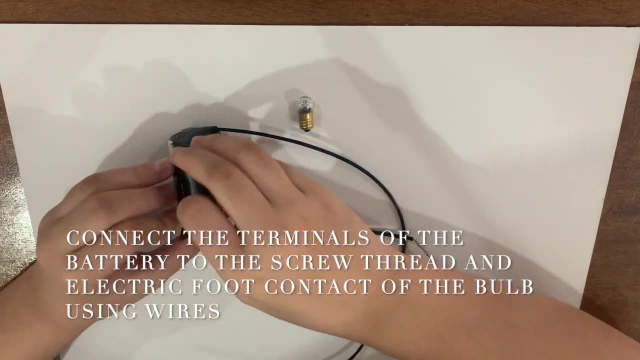 For a simple electric circuit, we need a battery, an electric wire, a bulb and a switch. For a simple electric circuit, we need a battery, an electric wire, a bulb and a switch. For a simple electric circuit, all you need to do is to connect the positive and negative terminal of the battery to the screw thread contact and the electric foot contact of the bulb using electrical wires. 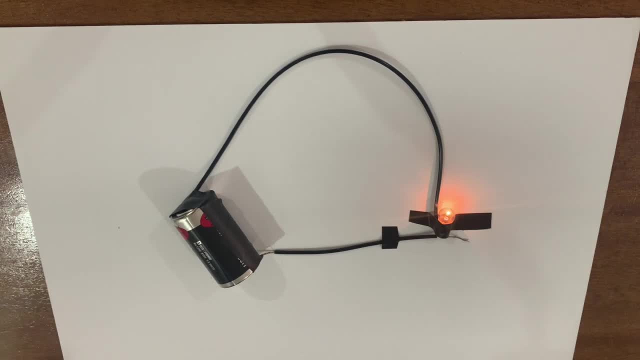 The circuit should look like this. You will notice that upon connecting the battery to the bulb, it will immediately light up. This is because the electrons can continuously move from the battery device. Now observe: If we remove one of the wires on any of the contacts on the bulb, the light on the bulb immediately turns off. 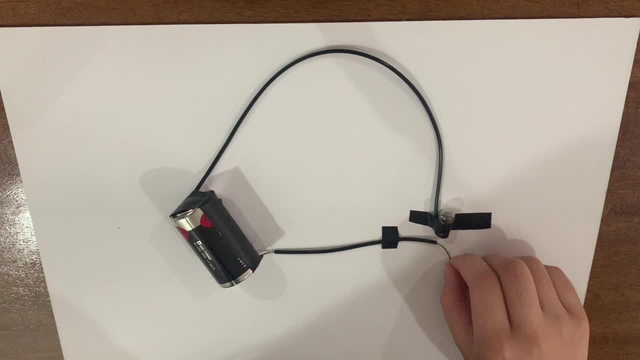 This is because the electrons can no longer flow, because the path it should be flowing was cut off. This is what we call an open circuit. This is what we call an open circuit. The current flows only through a closed circuit. If the circuit is broken, the current will stop flowing. 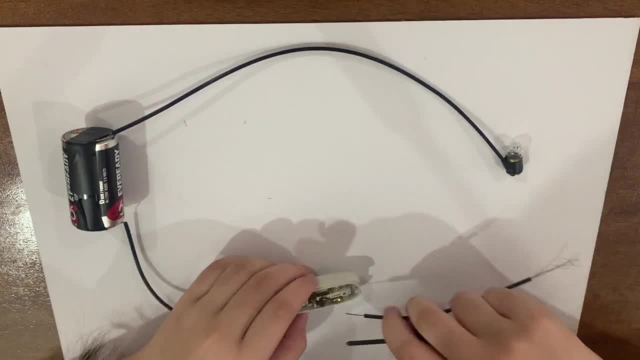 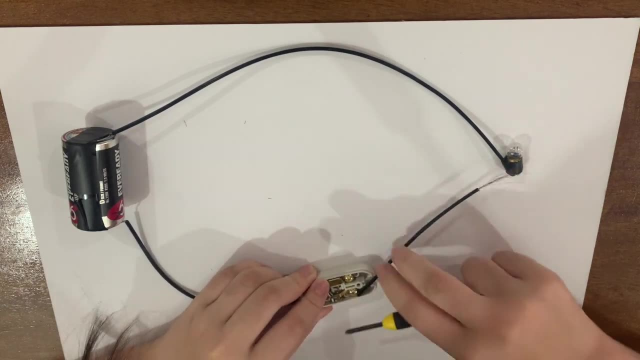 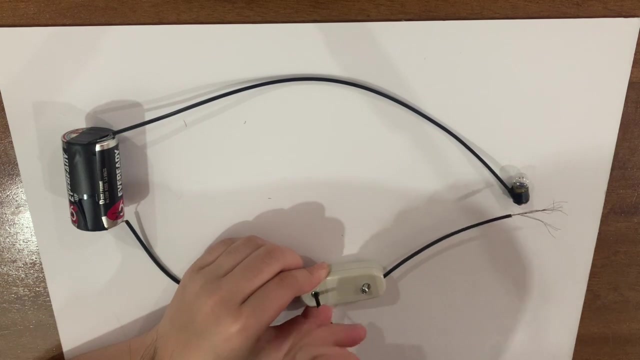 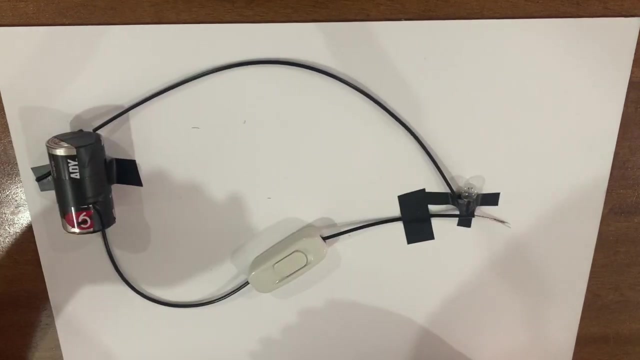 This is where a switch comes into use. A switch may be used to open or close the circuit. To add a switch on a simple electric circuit, we will attach the switch to one of the wires connecting the bulb to the battery. To replace the switch, we will attach the switch to the top LED of the light bulb. 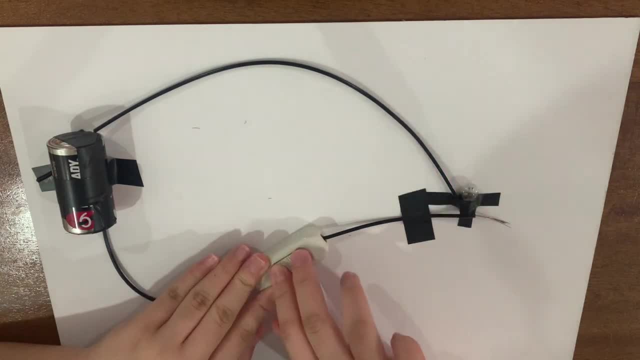 The complete set-up should look like this: If we turn the switch on, the bulb will immediately light up, And if we turn it off, the light goes into the qualics without eventually turning off the light. Thus, use the switch on the power control while using the electric switch to power the Repair gadget. 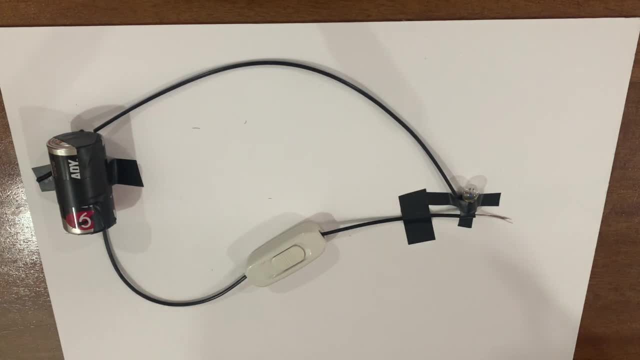 Thus use the switch on the power control while using the electric switch to power theanya light bulb at home meeting forms with electric bulb On some home desafory light Void lights, ya, so that we do not manually cut the wires or reconnect it in order to turn on and 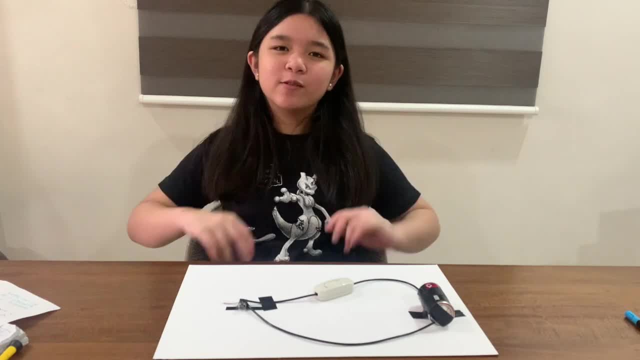 off our lights. Bye, bye, Thank you for watching. See you on our next project. 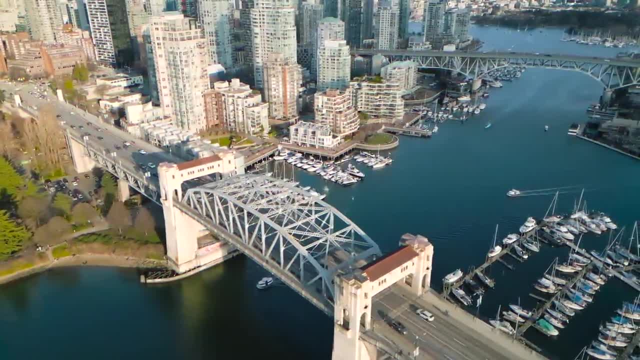 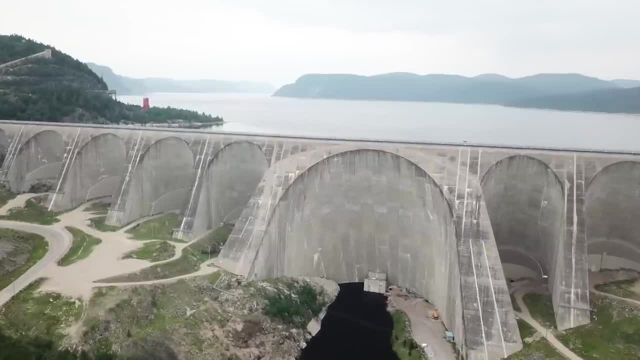 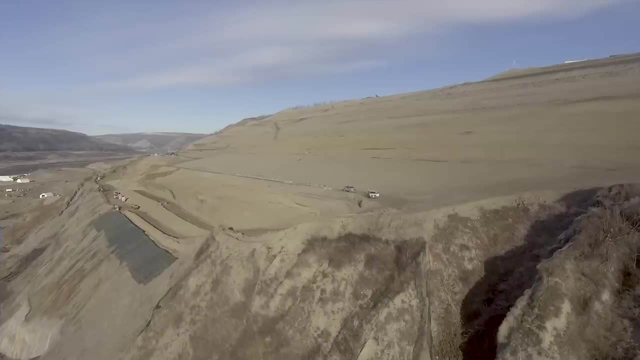 The British Columbia Province of Canada is a region well known for its exploits and awe-inspiring hydropower facilities and production. But amidst the rich history of power production stands a mega project of such magnitude that it has been dubbed the largest major hydropower project in the 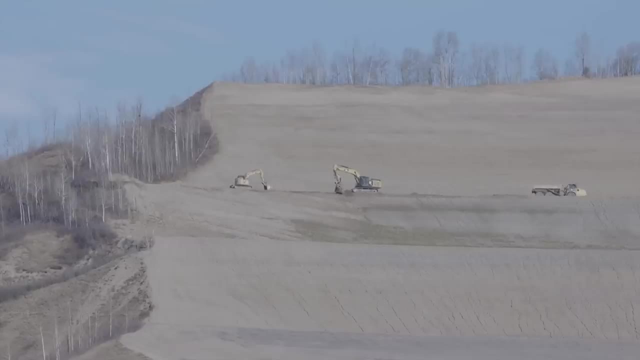 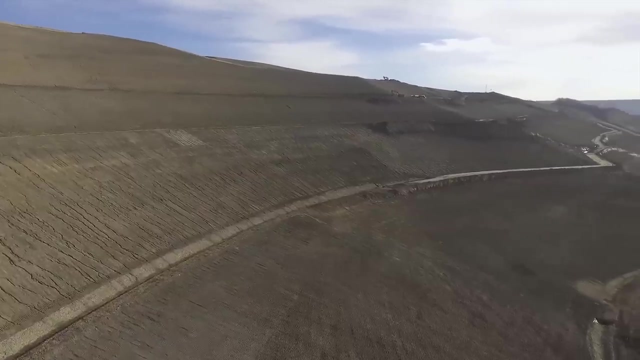 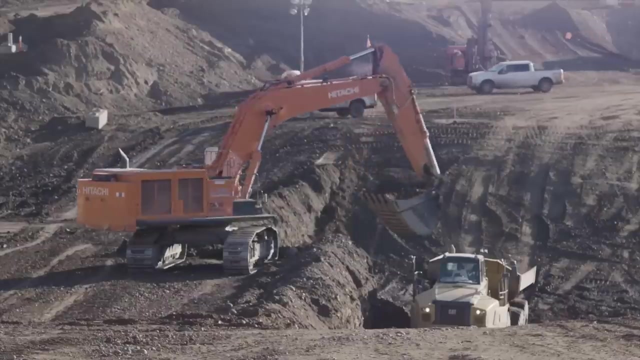 region since 1984.. Named the Site C Hydropower Project, it stands as the latest response from the province to the global push for renewable energy. This project is the newest addition to the already impressive history of hydropower generation in the BC area. Despite its 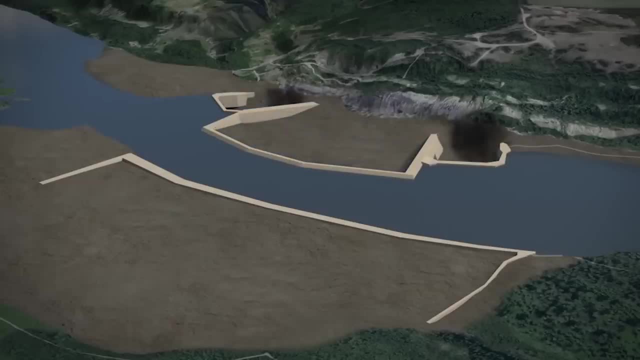 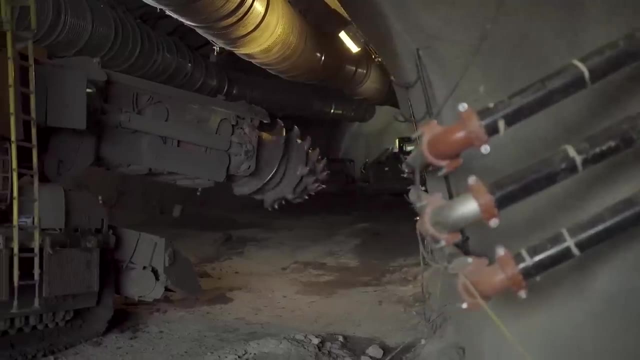 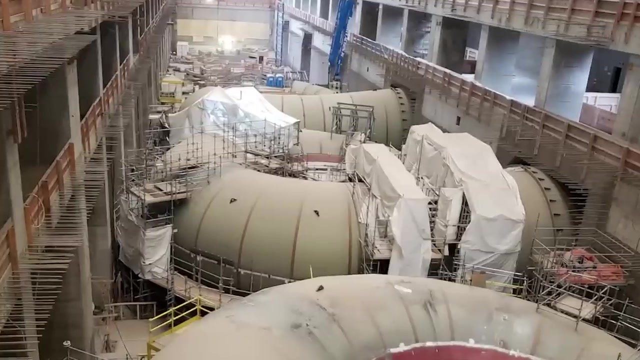 potential benefits. Site C is shrouded in controversies, leaving many to ponder what is the core of this bold hydropower venture and what changes will it bring to the region's power setup? Moreover, why does a station focused on renewable energy stir up so much debate? 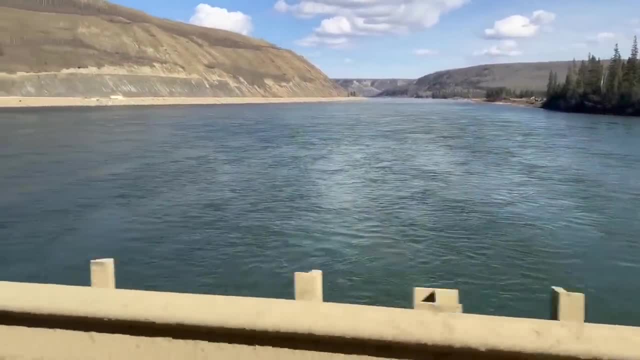 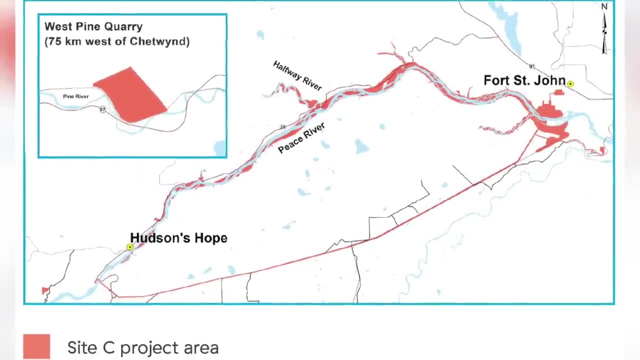 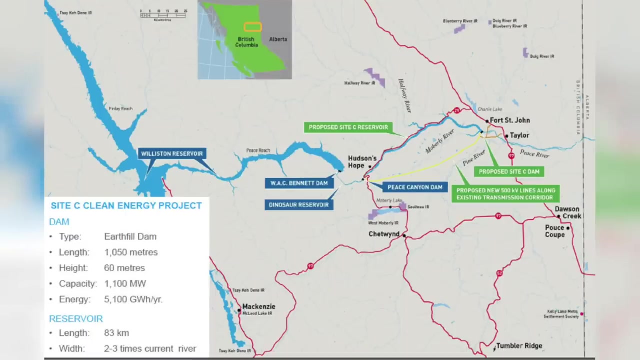 The Site C Dam is a major hydroelectric dam currently under construction by BC Hydro on the Peace River 14 kilometers southwest of Fort St John in northeastern British Columbia, Canada. The mega project is located approximately 80 kilometers downstream from the WAC Bennett Dam.